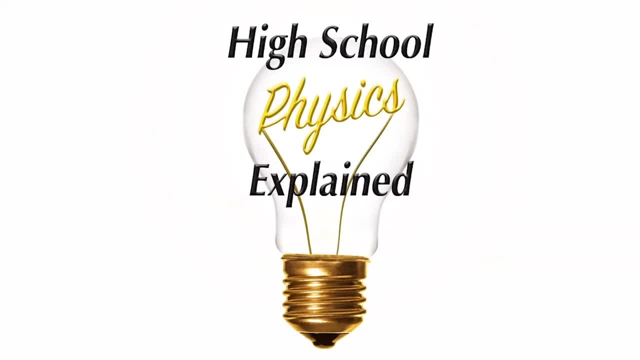 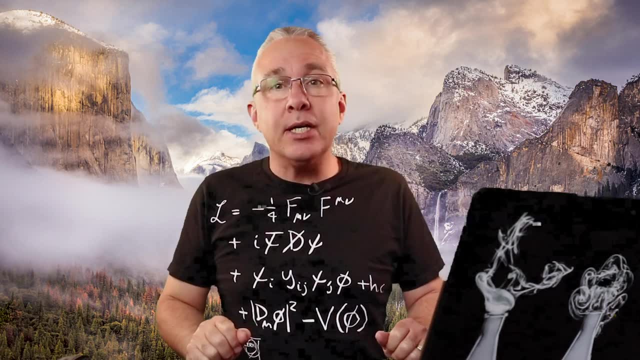 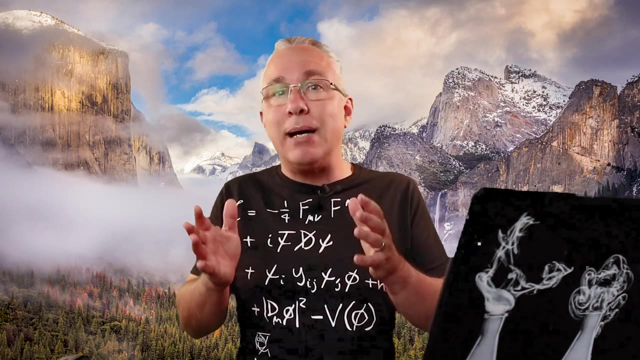 Now, what's the stuff all around us made up of? Now? it's a question that's been asked for thousands of years and throughout the millennia we've believed basically that matter around us is made up of basic building blocks and everything we see is simply a composite. 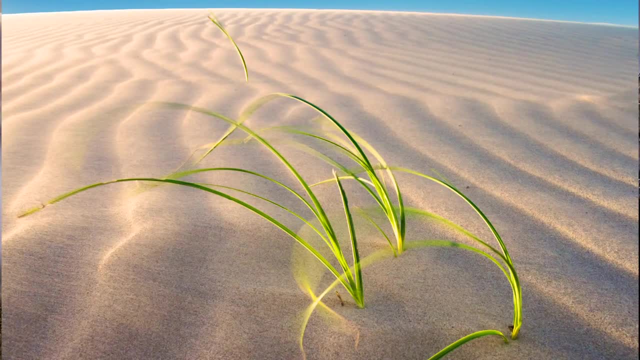 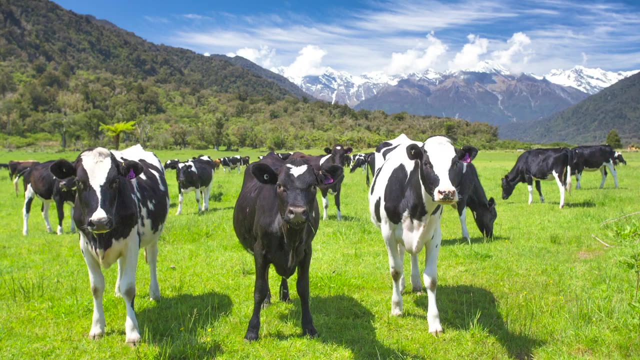 of something simpler, Whether it's the sand on the beach or the air we breathe or the water we swim in. in fact, right up to the most complex part of our universe, life itself, All of it, we believe, is made up of fundamental components. Now, Democritus, who lived around? 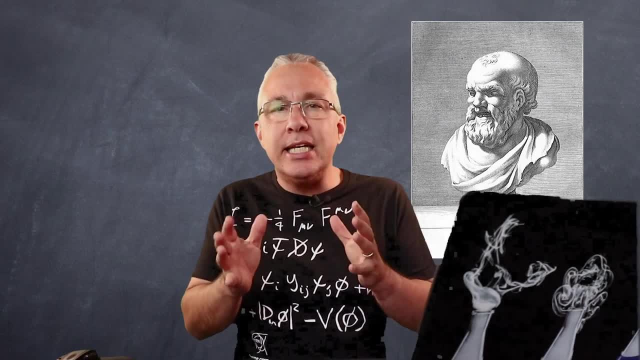 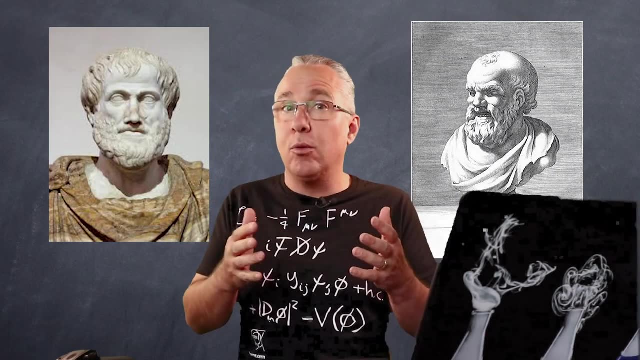 350 BCE, believed that all matter was made up of these individual particles, which he called atoms. Now Aristotle, who lived about 100 years after that, viewed that matter was made up of earth, water, air and fire. Although these views are models, both are markedly. 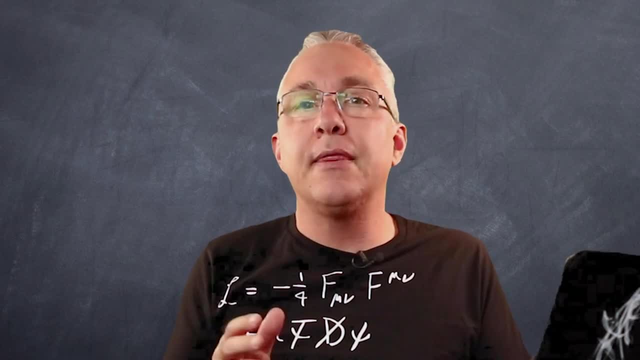 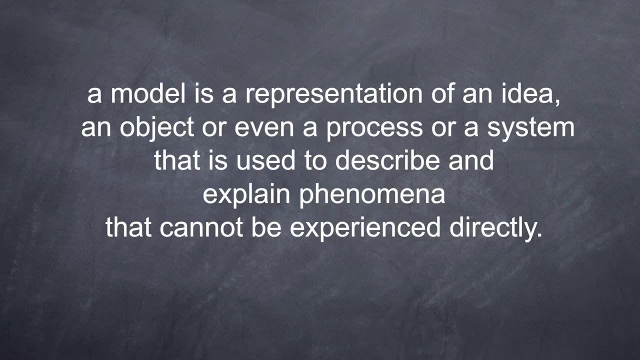 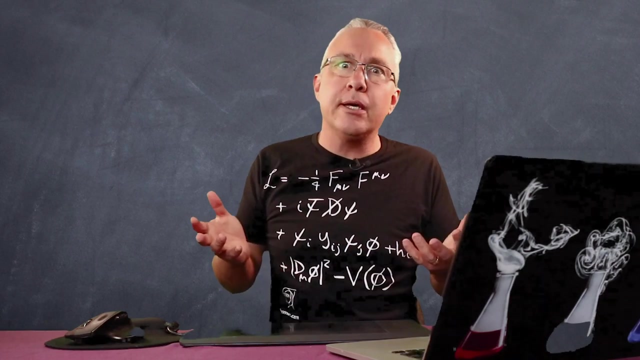 different, But they are philosophers and they did not test their models. So what are models Now? models in science are constructs designed to help understand how nature works, And that way of thinking- designing models and then testing them, refining them and, if necessary, throwing them out- is the hallmark of scientific investigation. 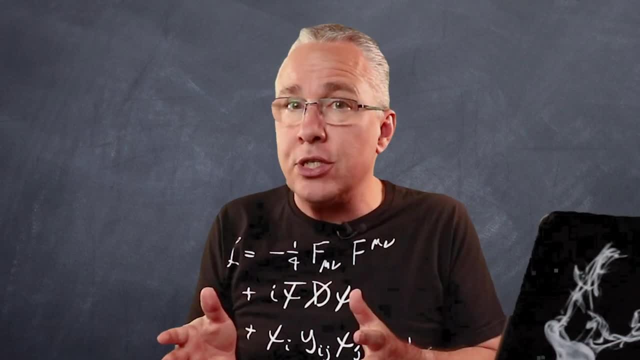 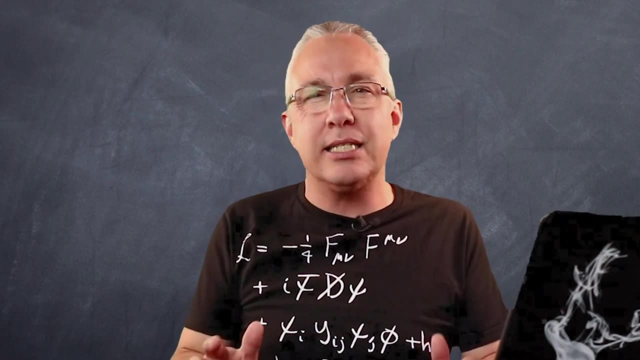 Now, importantly, models must be able to explain observations and be used to make predictions about new observations. So, strictly speaking, Democritus and Aristotle can't really make predictions and can't really be considered scientists, as they did not really test the 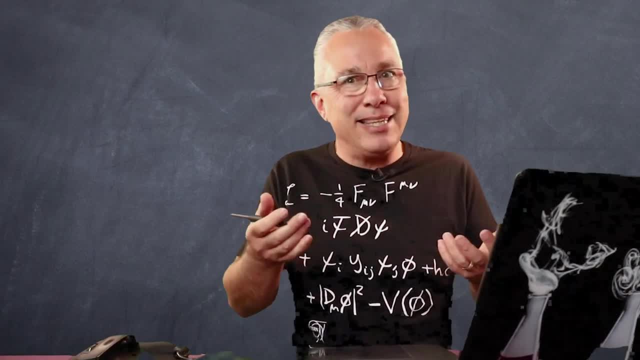 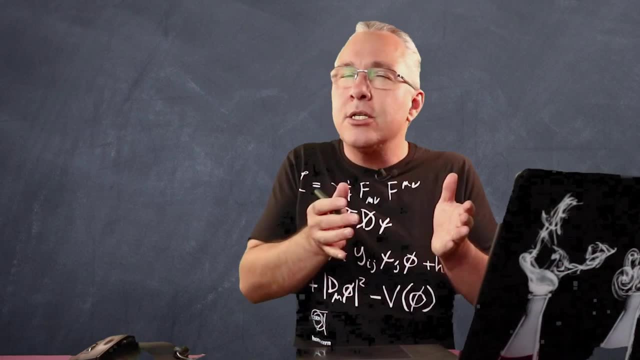 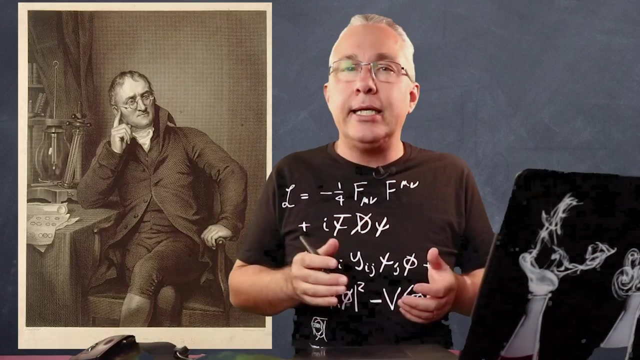 models they described. Now, this video is about the standard model of matter, So stay tuned. But I do want to provide a brief review of how we got to that model, so to accentuate how science actually works. Now, in 1808, John Dalton published his work on the atomic theory and he held the Democritus. 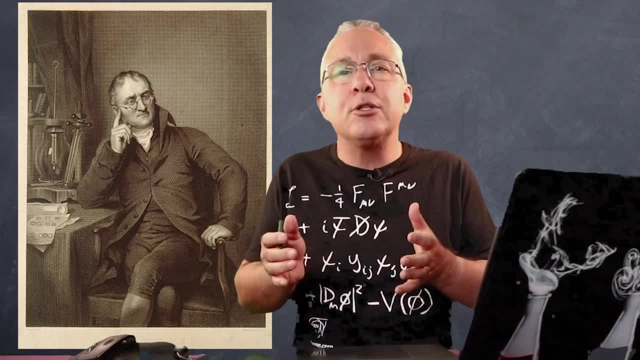 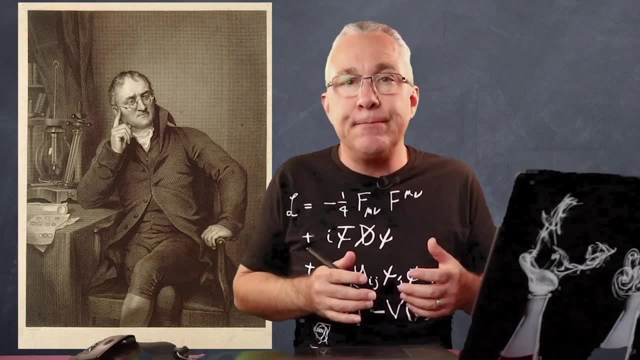 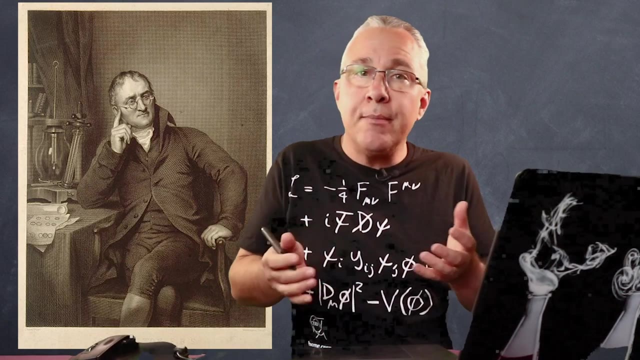 view that elements were made up of atoms. But he based on experimental work in chemistry and he greatly expanded that model. Atoms Of the same element were of the same size and characteristics And he came to the conclusion that chemical compounds were groups of atoms in whole number ratios and that chemical 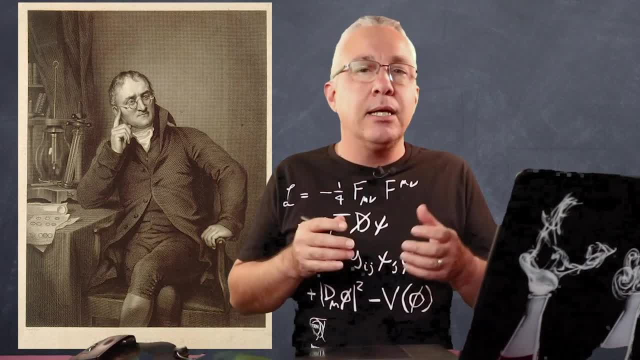 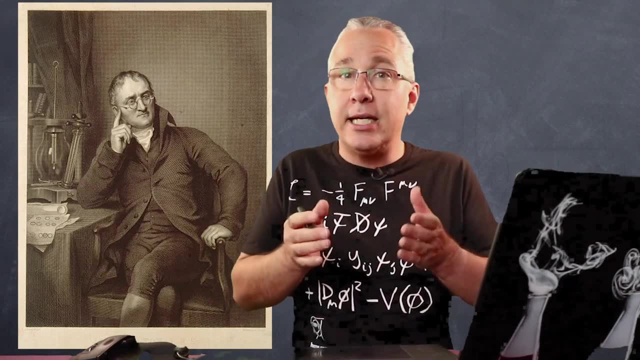 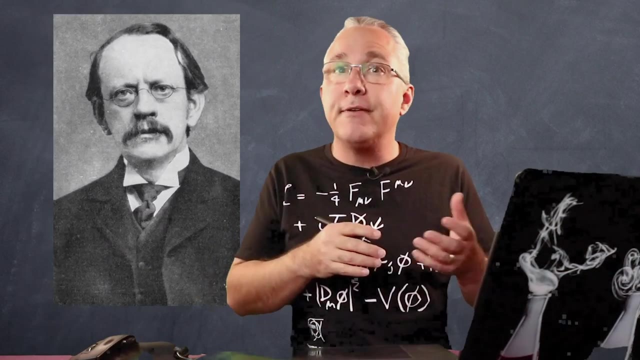 reactions were simply changing combinations of those atoms. Now his model is still true today and forms the basis of chemistry. However, one aspect of that model- that atoms are indivisible, as you will see- is false. In 1897, JJ Thomson, through a series of experiments to investigate the nature of cathode, 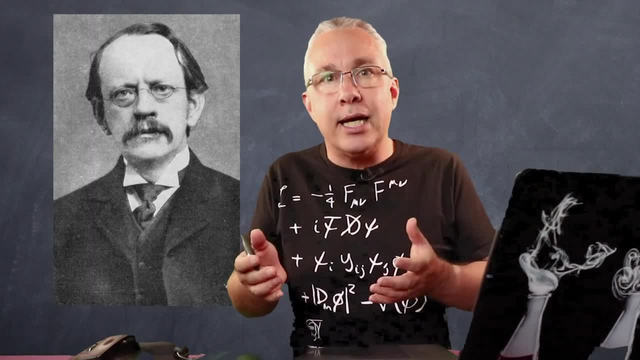 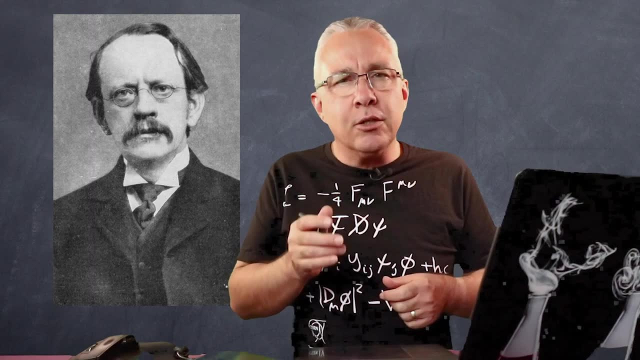 rays, discovered the electron and thus was able to explain cathode ray behaviour. Now you can look at the details of that experiment in my video link above. but he came to the conclusion that the model of the indivisible atom was incorrect. The atom was actually. 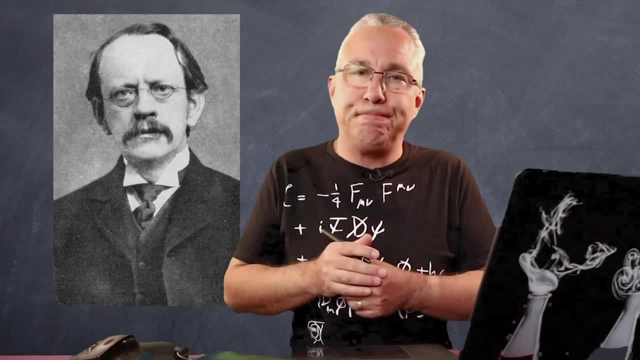 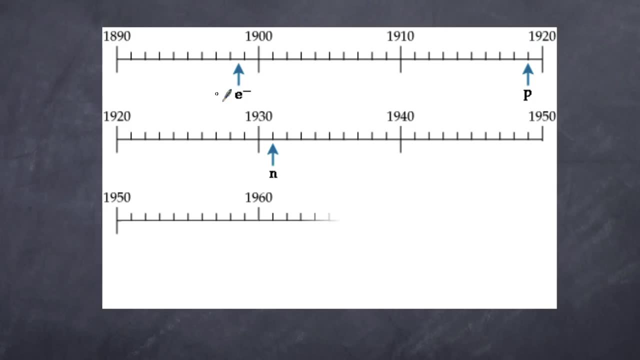 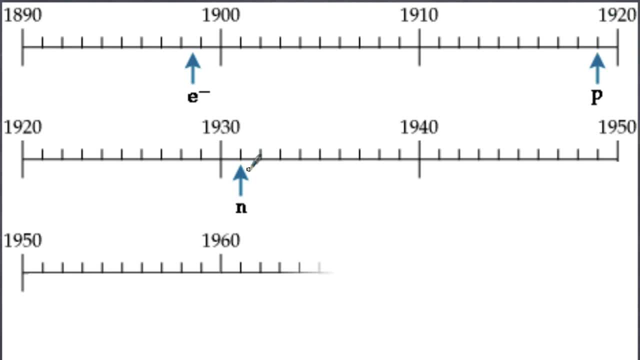 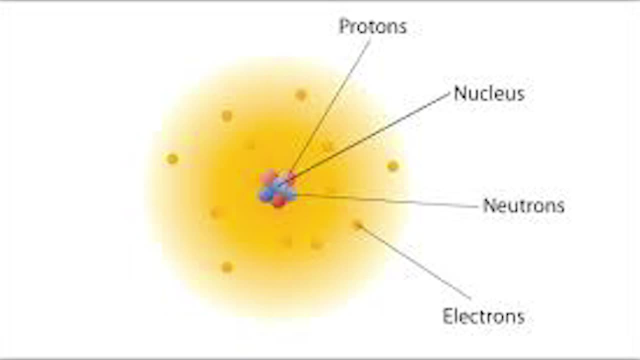 The proton was identified by Rutherford and then again in 1932 by James Chadwick, we have the discovery of the neutron. So now, by 1932, we have the model of the atom, basically made up of three components: The protons and the neutrons, which exist in the nucleus, and the electron, which in 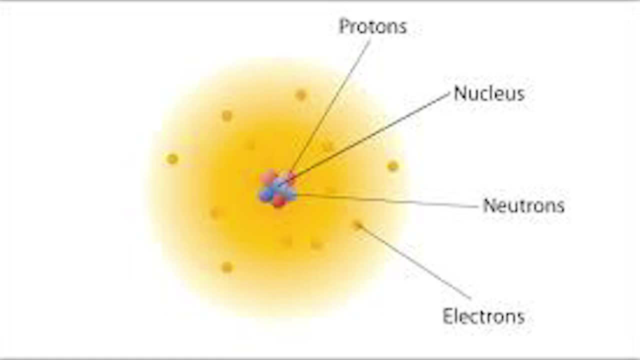 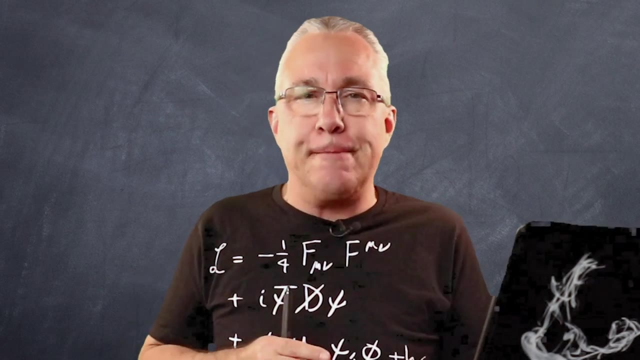 some form or another existed in orbit around the atom. Again, I do have videos in my Modern Physics playlist, so if you wish to explore those scientists further, check that out. The proton was identified by Rutherford and then again in 1932 by James Chadwick. 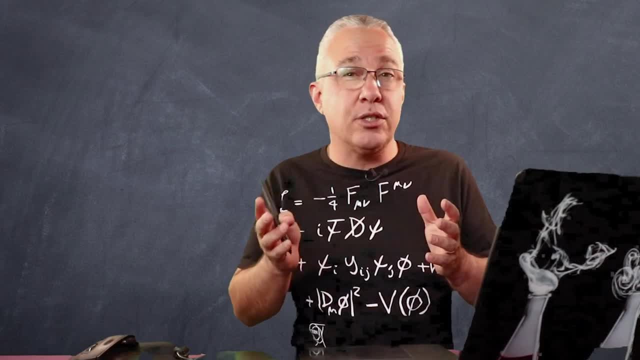 we have the discovery of the neutron. Again, I do have videos in my Modern Physics playlist, so if you wish to explore those scientists further, check that out Then. in 1930s, with the use of particle accelerators such as the cyclotron and the, 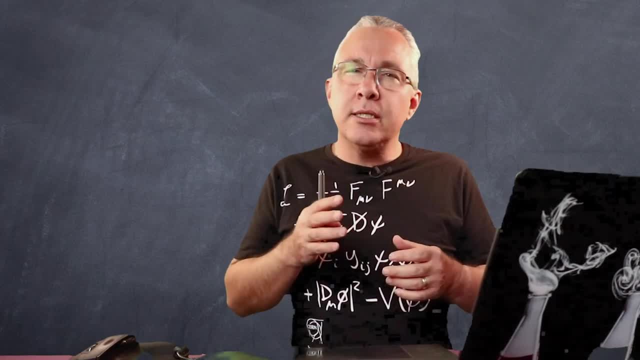 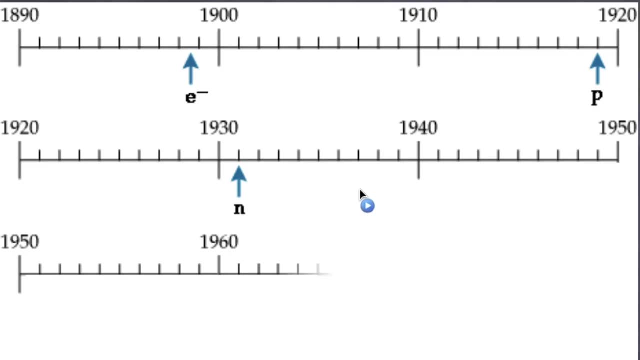 study of cosmic rays through bubble chambers. scientists continued to probe matter, to understand it better, To refine the model of the atom. But then, in 1937, we have the discovery of the muon Nowcking. that that, but we continue to have more particles. 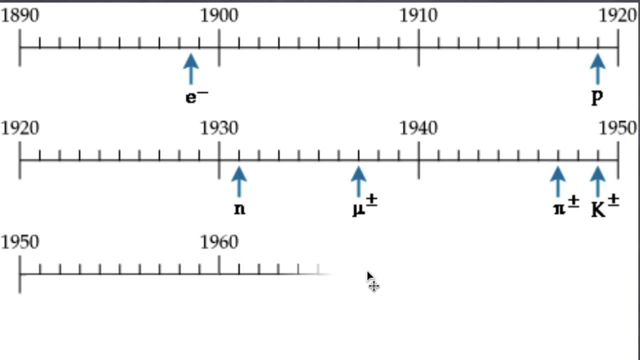 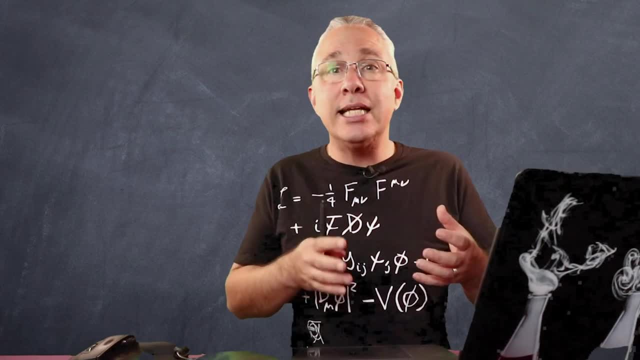 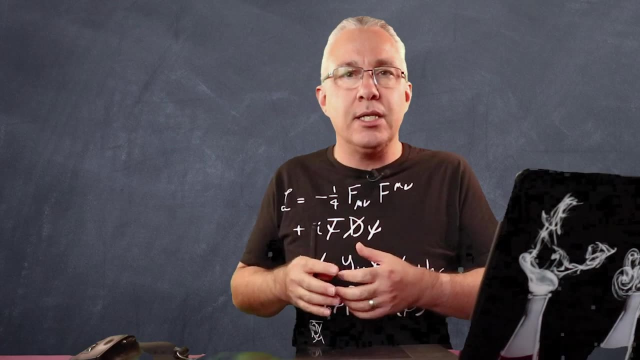 The Pion, the K-on, discovered in the late 40s. in the 1950s, a whole host of particles had been discovered. Each of these particles had its own combination of properties, charge spin. strangeness that all made them different to one another. And so now what we got was this: 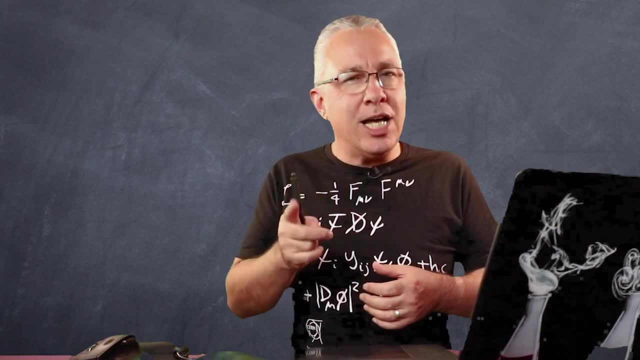 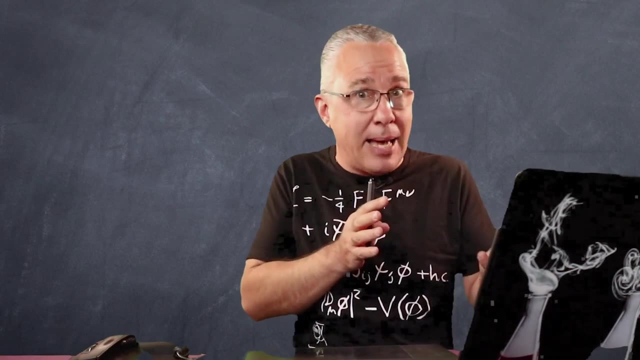 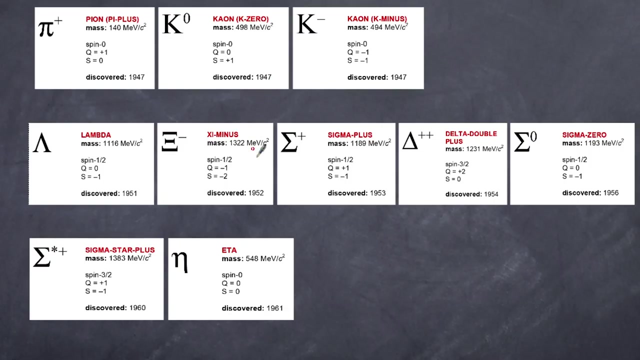 colloquially known a particle zoo. Now, charge may be familiar to you, and maybe not spin and strangeness, Don't worry too much about that. what they mean, except to say, like mass and charge, they are properties of subatomic particles which can be determined experimentally. So here is a selection of some of the 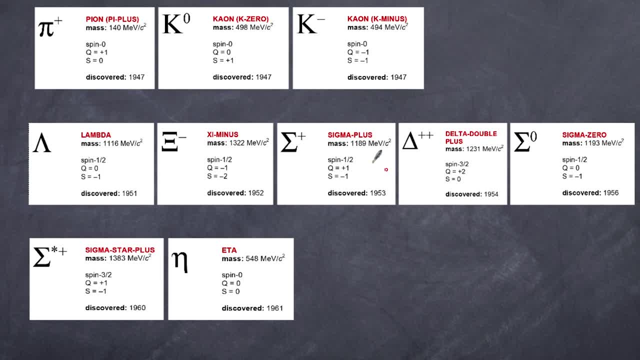 products were discovered in the 40s and 50s and 60s And, as you can see, each of the particles had a different property in terms of their spin, their terms of their charge and terms of their strangeness. None of this fitted in with 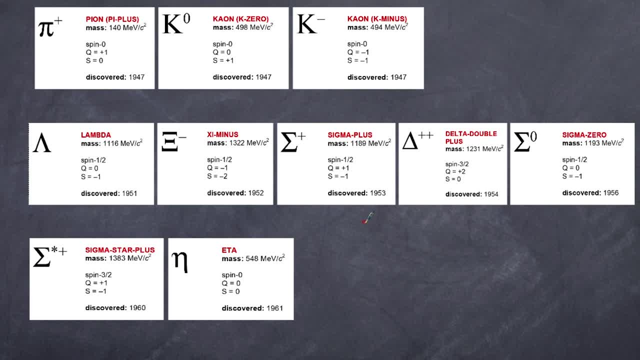 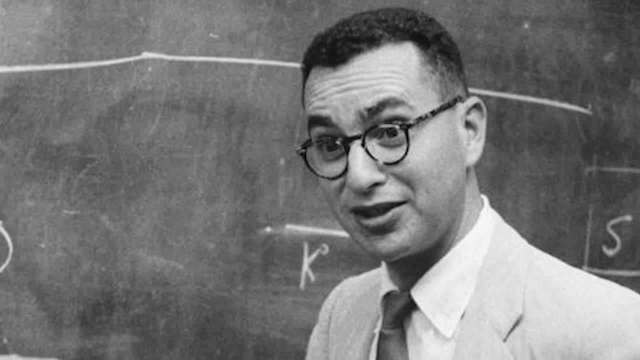 the current model of the atom, which at that time consisted of simply the proton, the neutron and the electron. So, in 1962, Murray Gell-Mann, believing that all these particles were somehow interrelated at a deep, fundamental level, that they were all made up of the same, 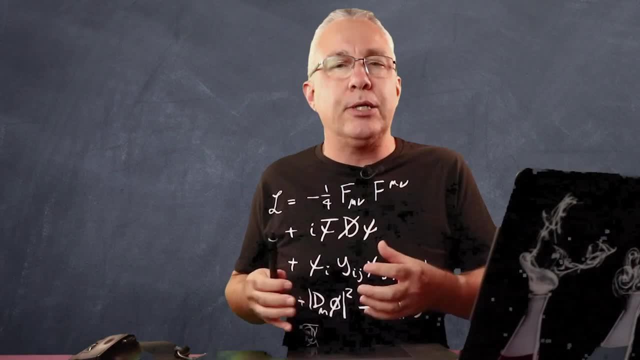 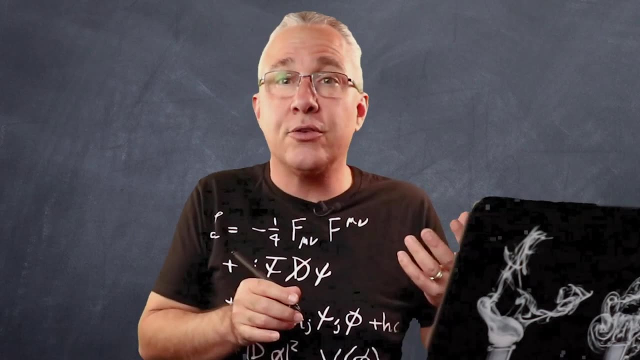 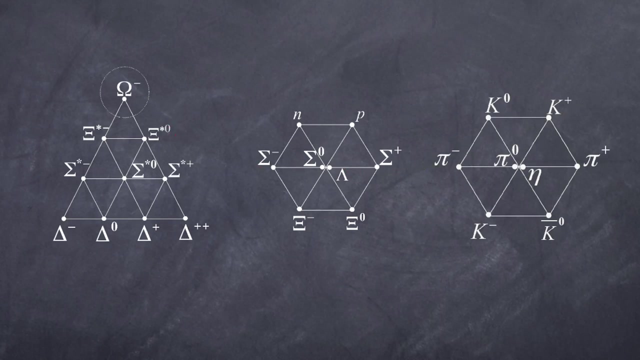 constitutions set out to build a model that could explain these particles. What he discovered? that if you arrange them according to their properties, that certain patterns appear, that it's triangular, And he developed this eightfold way. So here is a picture of the eightfold way that Murray Gell-Mann 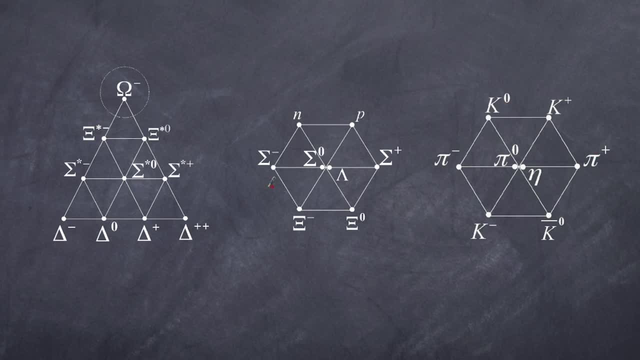 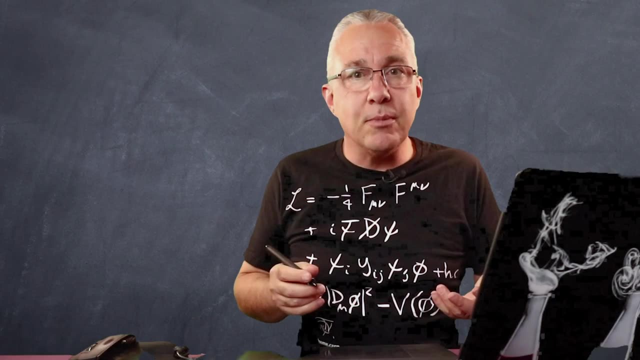 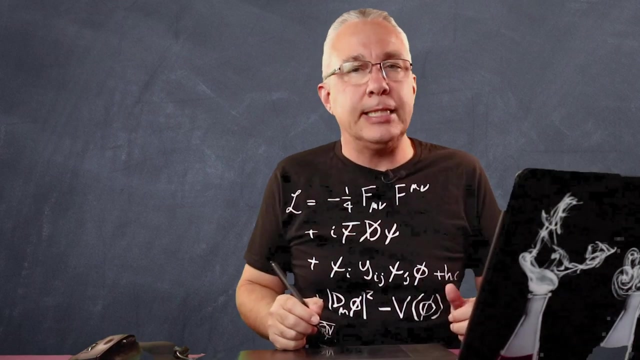 developed And you'll see, the particles are arranged in a way that relates to their strangeness, their spin and their charge. From this model he came to two conclusions. There was a missing particle called the Omega-minus, which he predicted would exist. Now this was missing in the known models, but he 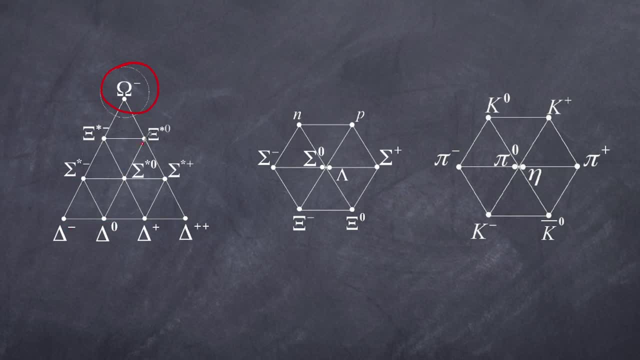 predicted that if we had four particles here, three here, two here and this was this other particle here which he was able to determine had certain properties to make it fit into this situation, In 1969 the Omega-minus was actually discovered and he got the Nobel Prize for. 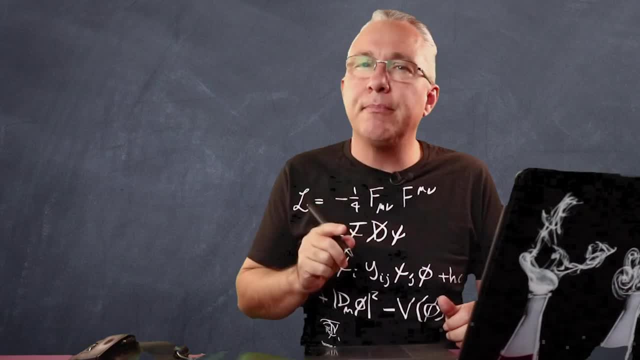 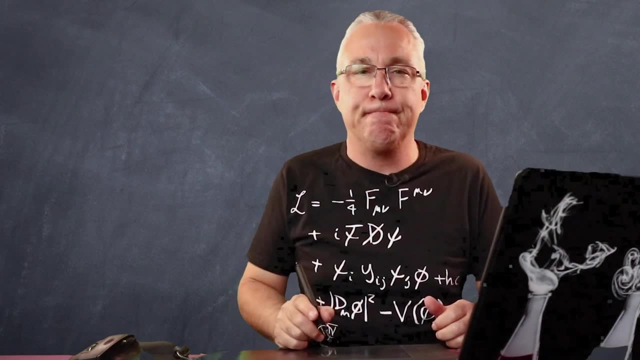 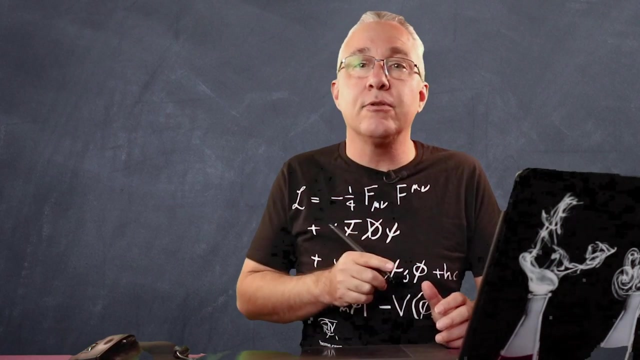 Physics that year. Secondly, the triangular shape pointed to the existence of three fundamental particles: the quarks, the up down and strange at the time. Now, this quark model proved to be very robust. Not only was he able to explain the existence of all particles that were there, but, with the addition of 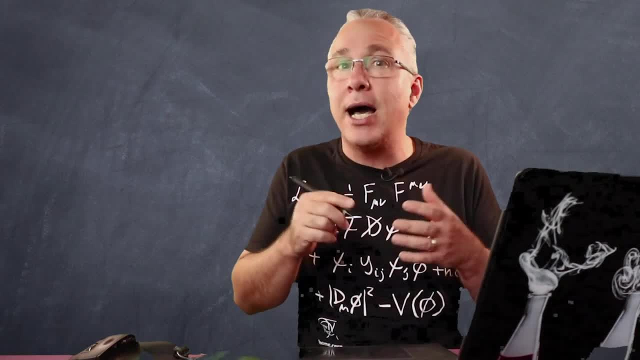 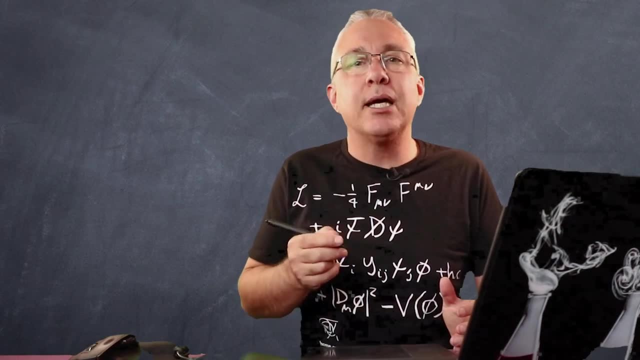 three other quarks, he was able to successfully explain the discoveries of other particles Since then. Now, his model has become known now as the standard model and it's become one of the most tested models in science. So what does this model look like? 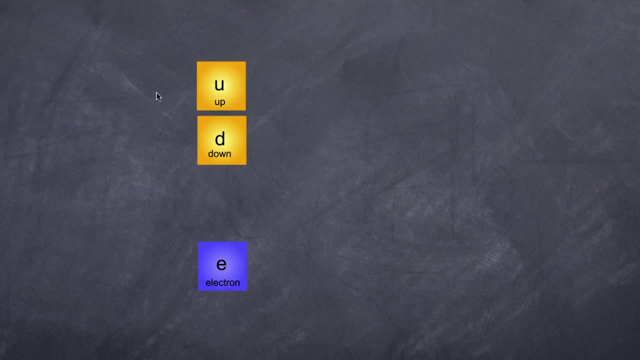 So let's start building our standard model. Let's first start by examining these two here, and these two things are what we refer to as quarks, And here we have two flavors of quarks. Down here we have an electron, and the electron is: 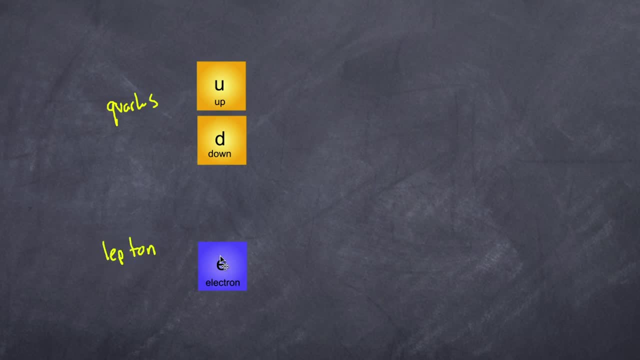 referred to as a electron. There is clearly forces that exist between these things. Something is holding these two together, and something is also responsible for interacting between our quarks and our leptons. So the first thing we have here is our photon, or our gamma boson. This is what we refer to as a boson, and it's 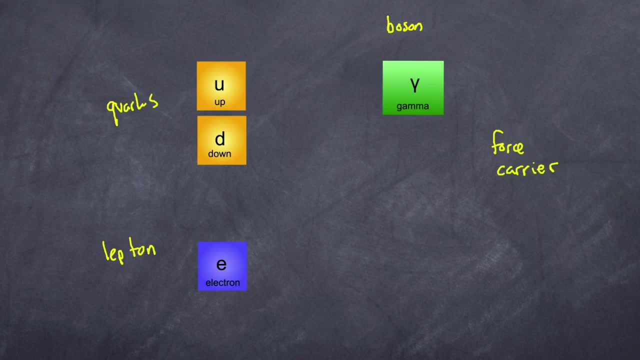 basically a force carrier. Now there is another force that's responsible for holding these quarks together, And that's a gluon. That's another type of boson. Now we know in radioactive decay that we may get a neutron convert into a proton, And when that happens- which we 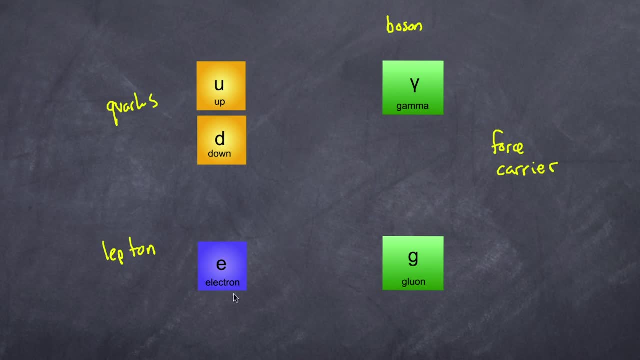 refer to as beta decay. we don't only get an electron emitted, so here's our lepton, but we also get a neutrino emitted, And this is also a lepton, a fundamental particle. Now, when a neutrino is emitted as well as an electron, there's some sort 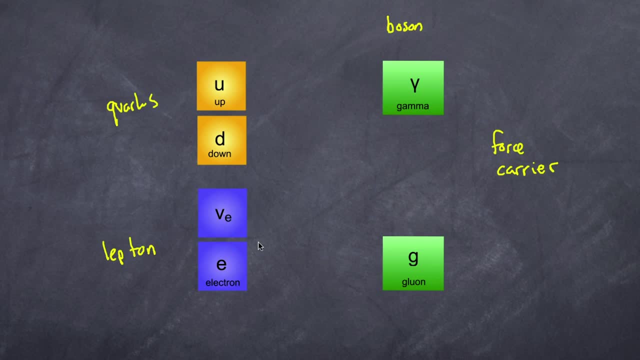 of force that's responsible for holding this all together beforehand, And these are our bosons, called the Z boson and our W boson. So now we have four bosons that are responsible for carrying forces between the quarks and themselves and quarks. 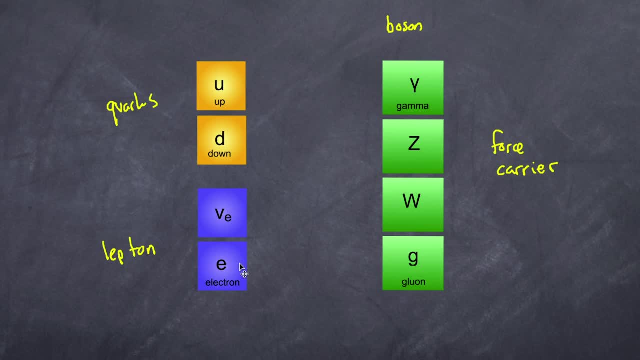 and the leptons, But here is one generation of particles which we're now going to be called our fermions, And we've since discovered that there are actually not one generation, but actually another two generations, each with their own couple of quarks, their neutrino and their muon. So what we now have is six. 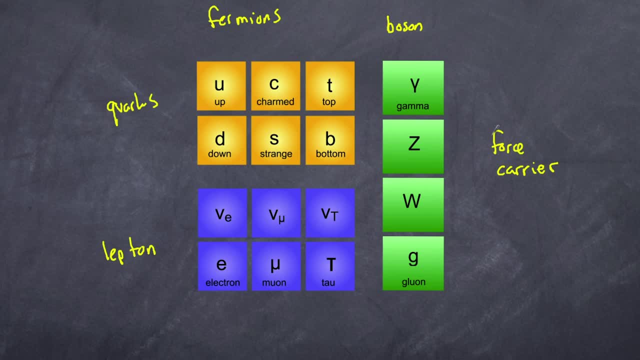 flavors of quarks. The top row of quarks all have a charge of positive two-thirds. Our next row of quarks all have a charge of negative one-third. Now, before you worry about fractional charges, it's helpful to know that the value of charge 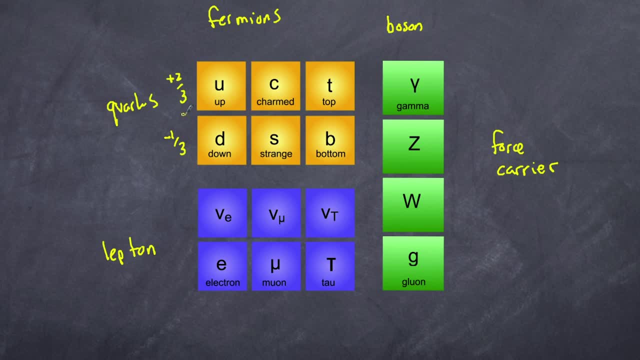 of plus one and minus one given to our protons and electrons is just being an arbitrary number. It's simply a label. So in order to understand the nature of composite particles such as protons being made up of quarks, we have to give these quarks a fractional value of those. 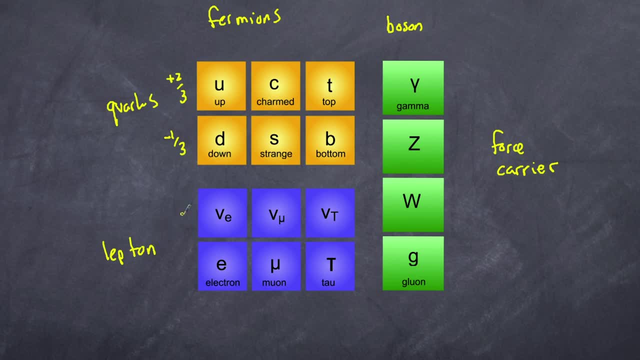 particular charges. Now, in terms of leptons, the charge for our neutrino is zero and the charge for our electron is negative one. So what I'm saying here is that the up, charmed and top are all quarks, all flavors of quarks, And the only thing that differs 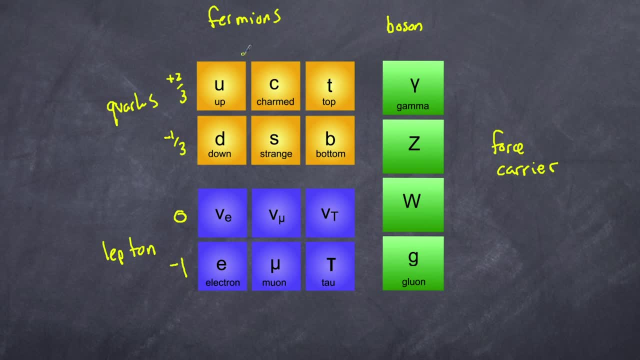 between the up charge and top quarks is the fact that we have an increasing mass going from left to right. This is true also for the down, strange and bottom. This is true for the neutrino. Now E means it's the electron neutrino, but we 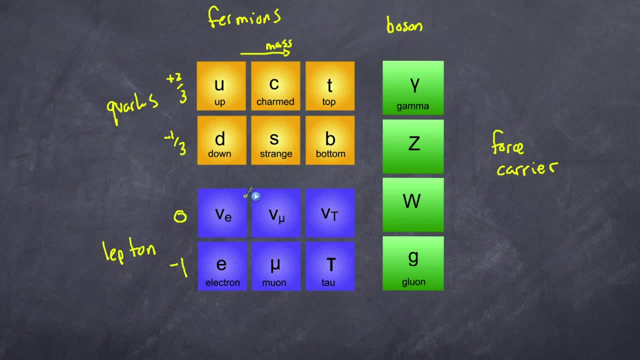 also have the muon neutrino and the tau neutrino. Each one is slightly heavier than the previous one. So we have fermions here broken up into quarks and leptons, and then we have bosons. Now, the strict definition for fermions is that they have a spin of a half integer, whereas 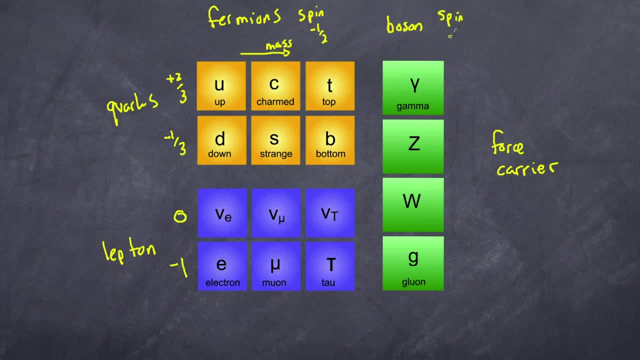 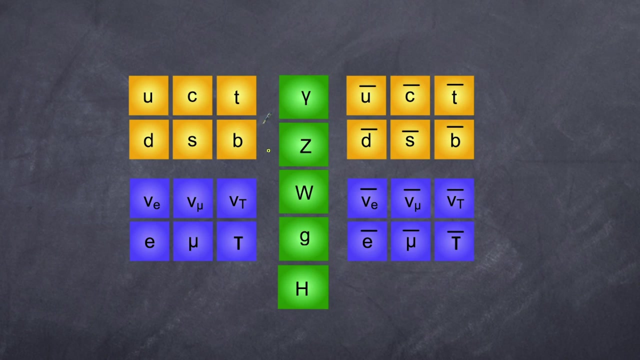 your bosons have a spin, In other words, at certain intervals they may spin up in wp values. So we can say that we have one half integer that corresponds to 8, a half a quarter of a value of one. Now that's actually only one half of the standard model, Because we now know also: 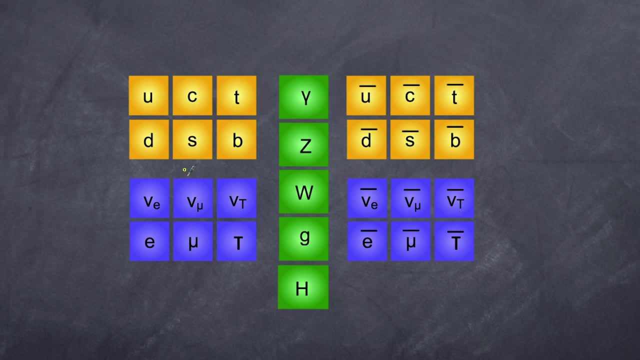 and then we have here is what looks to be a mirror of the other side, except this bar, and all these bars are your anti material. so we have your anti up quark, anti charmed quark, anti top and so forth. so all of these can be simply. 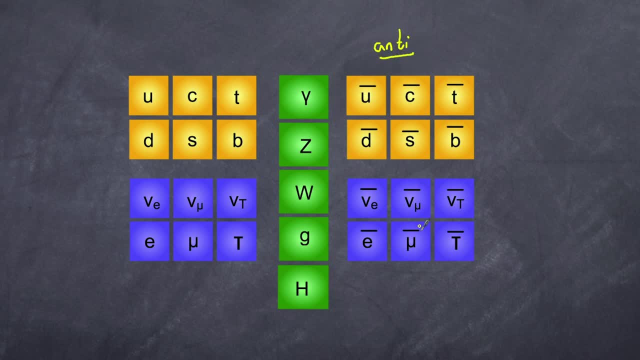 labeled exactly the same but just with the word anti before it. in this case the properties change just slightly. so, for example, our electron here has a negative one charge, but we know that our anti matter version has a positive one charge. it is opposite in charge in terms of our up quark. we know that is a positive two. 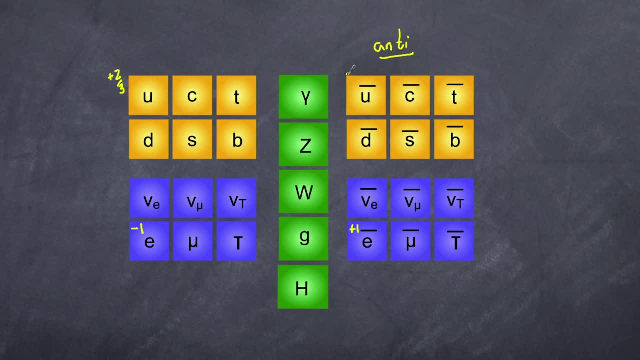 thirds charge. well, our anti up quark is a negative two thirds charge. similarly speaking, we have negative one third for this row. this becomes positive one third for this row, and so forth. obviously, this is still zero. you can't have a negative or positive zero, so that 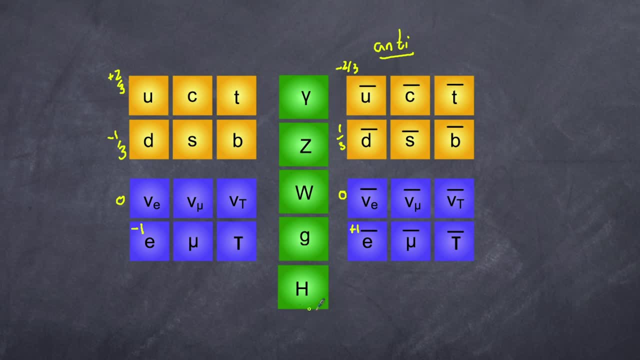 is in essence our model, but you'll notice here I've also included this H. what's this H? well, it is the Higgs boson, and the Higgs boson is the particle that was postulated in the 60s by Peter Higgs to be the force carrier in terms of them. 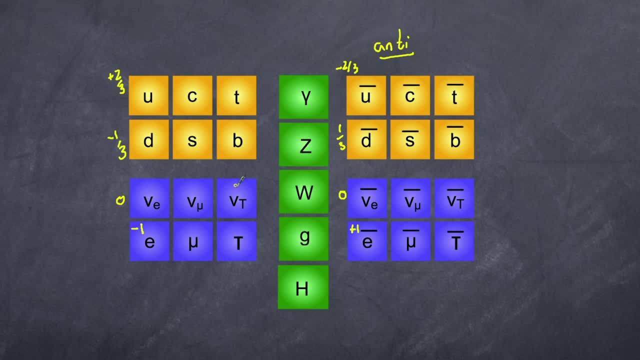 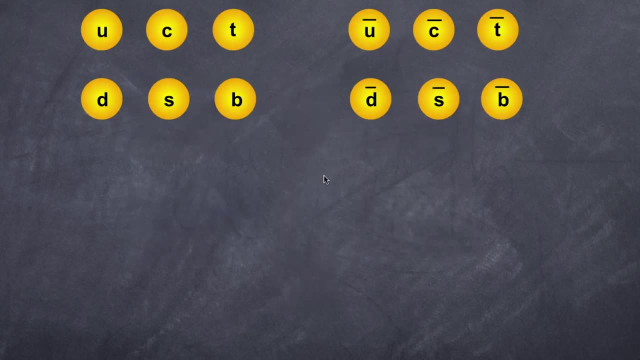 but contributes to the mass of our quarks and, of course, through the experiments at CERN, it was actually determined experimentally in 2012. so let's put us all together and let's see if we can make a number of particles by combining the number of quarks together and essence. a hadron is a. 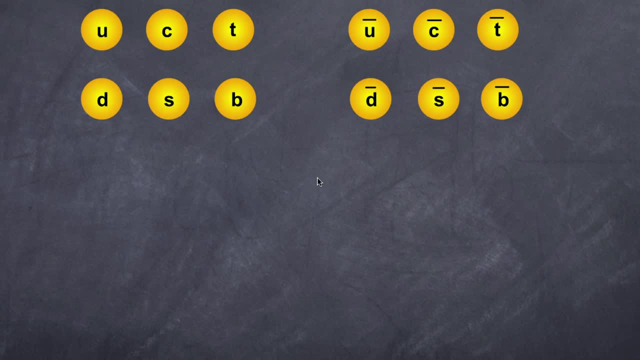 particle made up of multiple quarks and we can divide those padrons into two camps. they can be a baryon made up of three quarks or a meson made up of two quarks, but there are some couple of rules that we need to follow. let's first 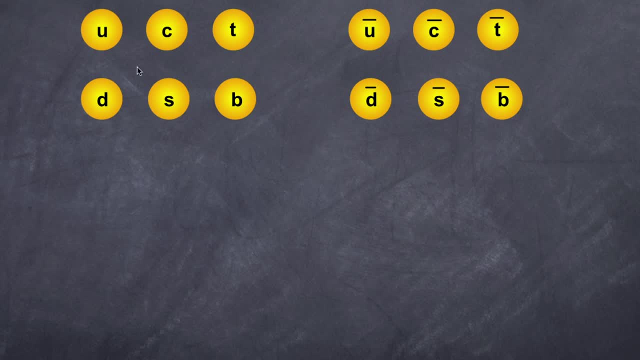 make up our most familiar barrier, and that's a proton. and a proton is made up of two up quarks and a down quark. now, what holds this all together? that is the interaction between things called gluons. so I'm going to add a couple of gluons. in fact, there are many, many gluons within. 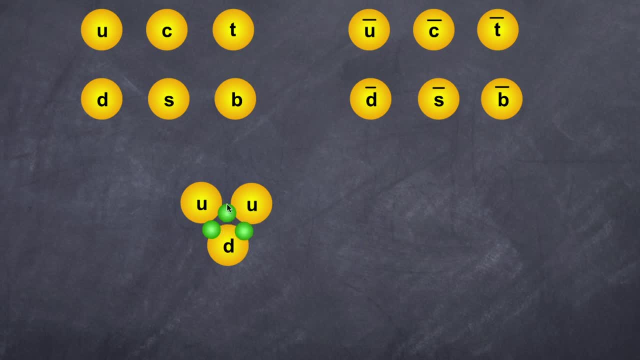 what we call a proton. but I'm going to put here three and it's an interaction between our ups and our down. if I were to look at the charge, we know that the charge of our ups are positive two-thirds, and of course two-thirds here, and our down is a negative one-third. if you combine that, you can see my charge. 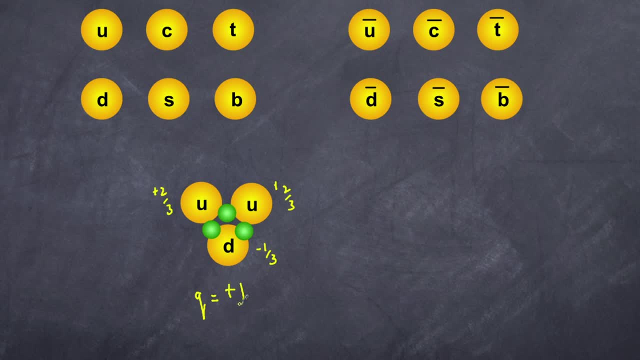 now is going to be a value of positive one, which is what you know: a proton exists now. the fact is is that there's repulsive forces between our ups and attractive forces between our downs, and that's, of course, an electromagnetic force which is carried by our gamma photon or a gamma boson. but we know that. 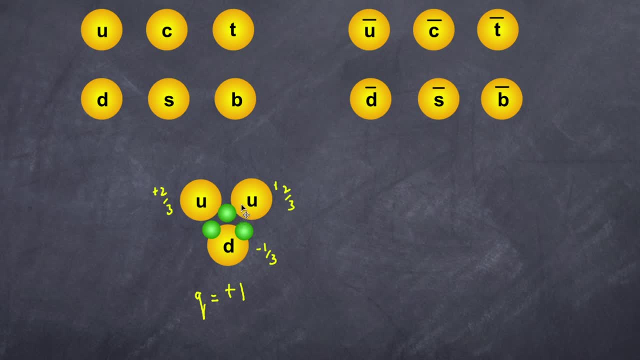 our gluons are much, much stronger in close range, and so, therefore, we'll hold this all together, but they are only effective at short ranges, so there is a boundary at which this can actually be existing. that is, beyond this dotted line, so to speak. the forces of the gluons will be too weak, and the 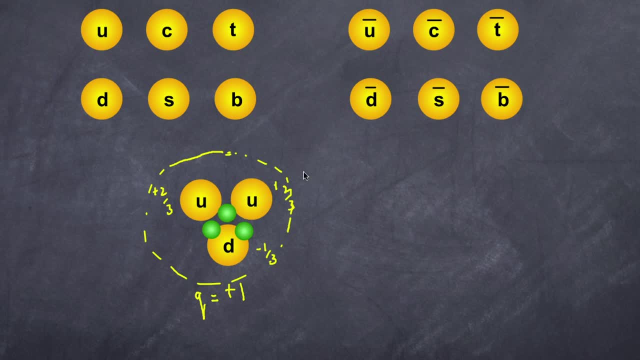 proton will fall apart. so the proton isn't a ball, it's actually a basically a sphere. these things are just a sphere and they're not a ball. they're just a sphere. these things are fundamental particles. they are, so to speak, points where these can exist within this particular volume over here. so there is. 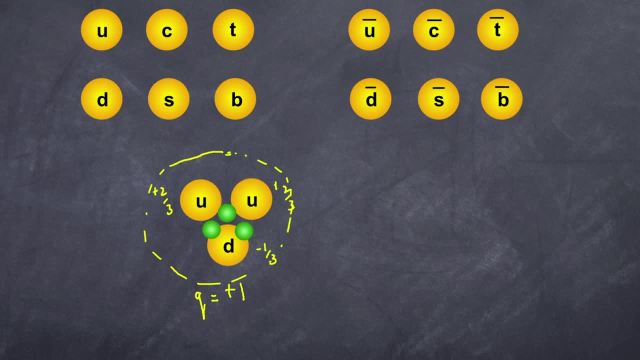 our proton. but can we make something else? how about we make a lambda? or what's a lambda? a lambda is made up of an up, a down and a strange quark now, because my up is positive, two-thirds, and my down is negative a third and my 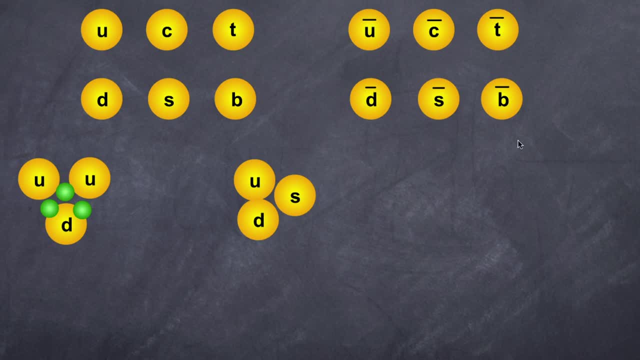 strange quark is positive two-thirds and my down is negative a third and my strange is also a negative third. then this has a charge of zero. so this particular barion- again it's made up of three quarks- is actually neutral, and this is our lambda, and it's often written like this. but now let's make something. 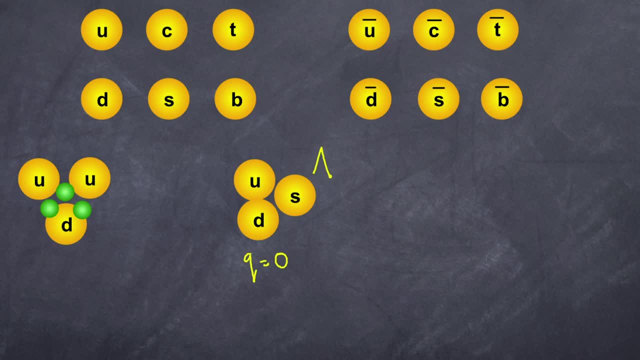 completely different. let's make a meson now. a meson is not made up of three quarks, it's made up of two quarks but, more critically, it's made up of a normal matter quark with an anti-matter quark. so, for example, i could have, let's say, 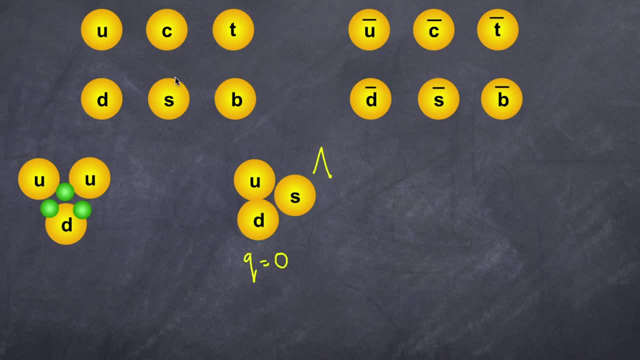 the kaon, and the kaon plus in this case is going to be my up and then my anti-strange, and so now we have a charge here. up is two-thirds. anti-strange, remember, now- is not negative one-third but positive one-third. so now what we have is a charge of equaling plus. 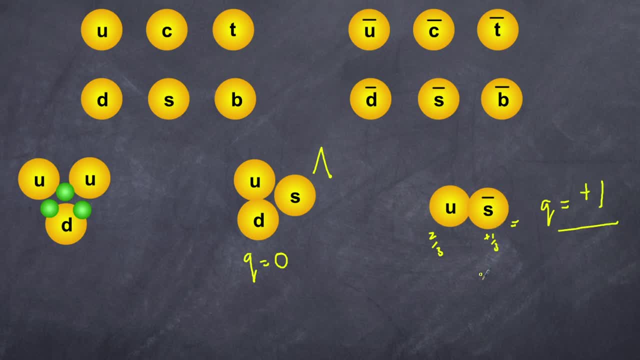 one, but it's only two quarks, so we call this now a meson, where this here is a barion, but both of them are referred to as hadrons. all the other known particles can be explained using this model in the 70s and 80s through accelerator work at 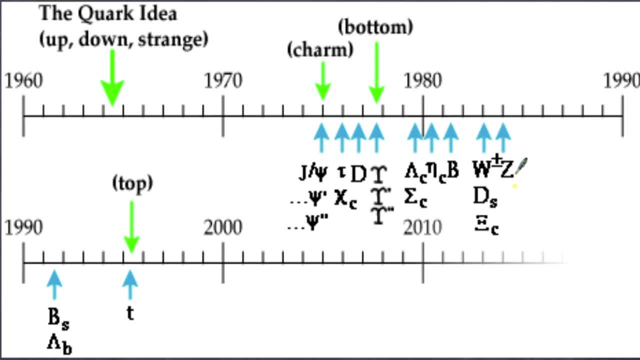 CERN and Fermilab and others. we discovered a whole host of particles that can all be verified using my gelman's standard model. as you can see, some of the particles that we've discussed are already here. now we have all of these terms here, but just to make 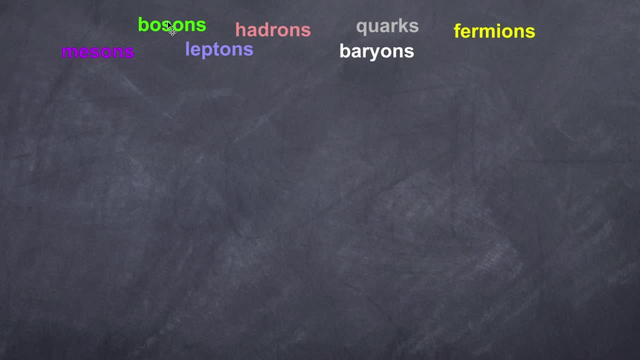 it really clear. how do they relate to each other? now, remember, we can divide all particles basically into two groups. the first is the bosons and the second are the fermions. in essence, bosons and fermions are separated by the fact that bosons have a spin of equal to one and fermions have a spin of one. 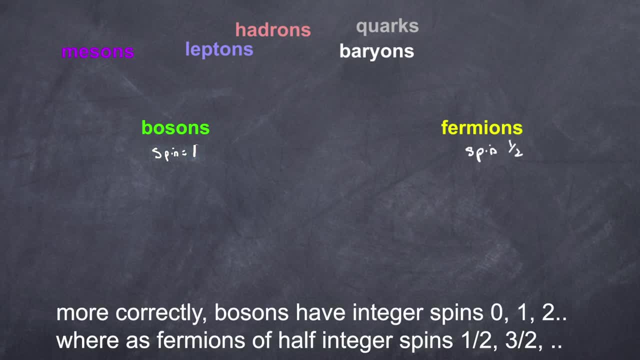 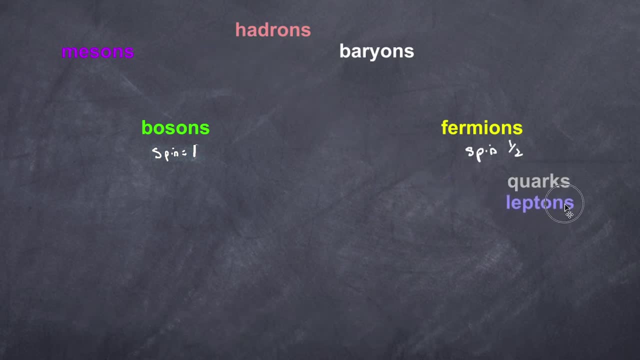 equal to half. now that means our quarks are going to be in the fermion aspect as our leptons on this side here Now. our bosons include, of course, gluons, our W and Z and of course our Gamma, but bosons don't have to be fundamental particles. 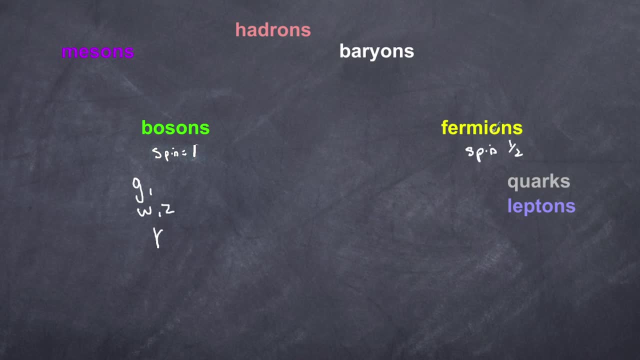 fermions don't have to be fundamental particles. as long as it has a spin of half integer, it can be one-third, can be a fermion And baryons, as a result can be fermions that, because they're made up of three quarks, will always have a spin of a half. 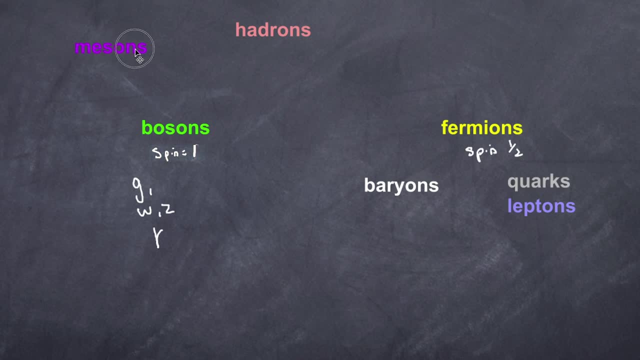 integer Mesons because of their nature, that is, a combination of a single quark and a single antiquark, will always have a spin of zero, So there can be a boson as well. So you have now two types, fundamental ones and composite ones- in. 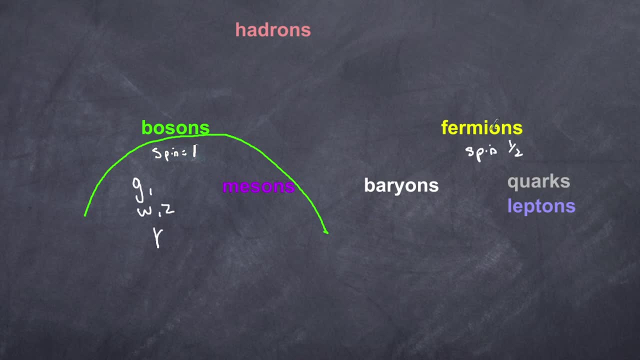 this case our mesons, Our fermions, can be divided up into two types: a composite of baryons and our fundamental ones, which are your quarks and your leptons. Your hadrons, by their very definition, are made up of multiple particles. So